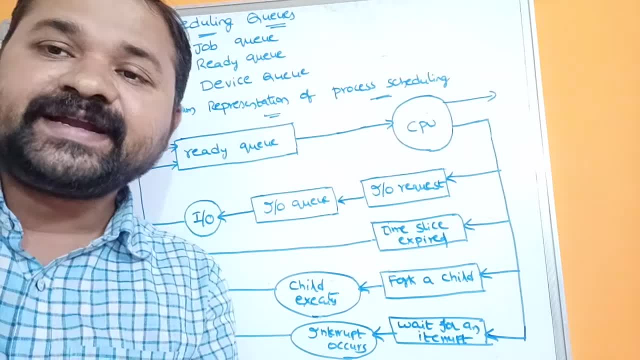 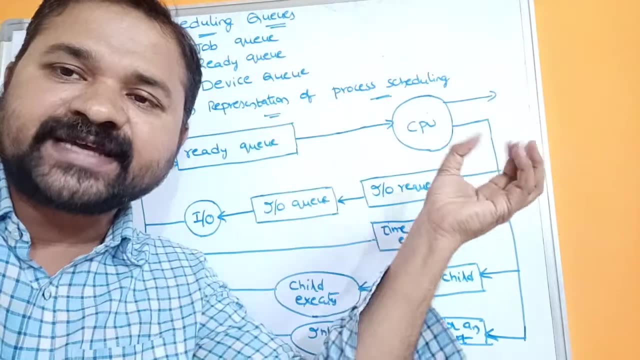 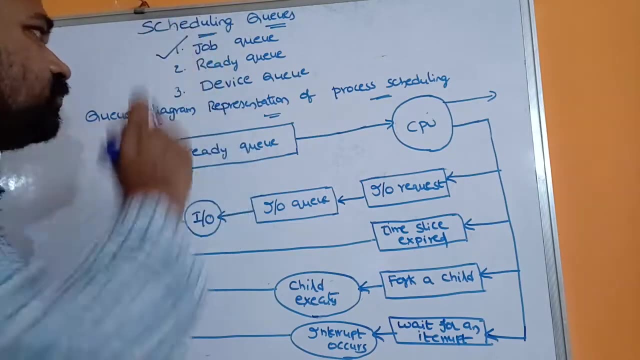 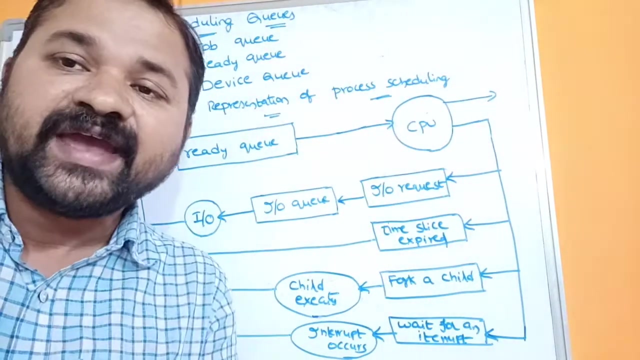 So that is about what is job queue? Job queue contains list of all the processes which are in the system, And job queue resides in secondary memory such as hard disk. Now let us see about the second one, that is, ready queue. Ready queue contains list of all the processes which are waiting for execution, which are ready for execution by the CPU. 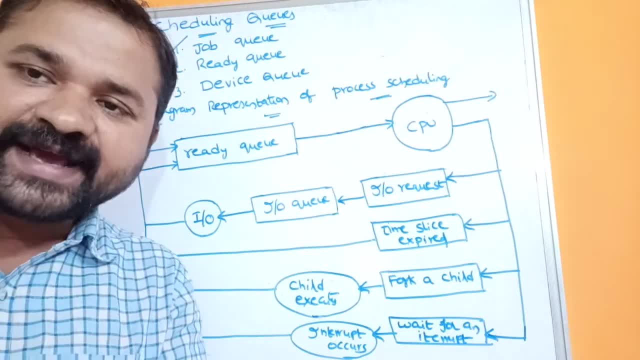 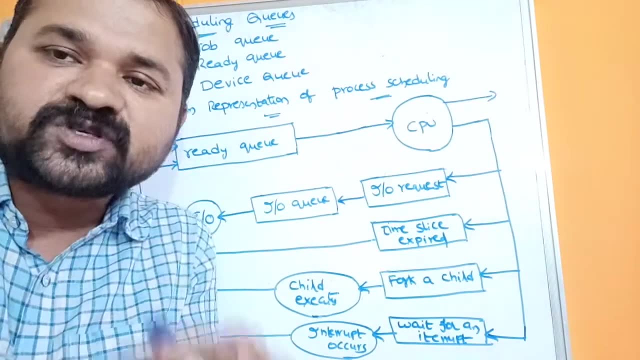 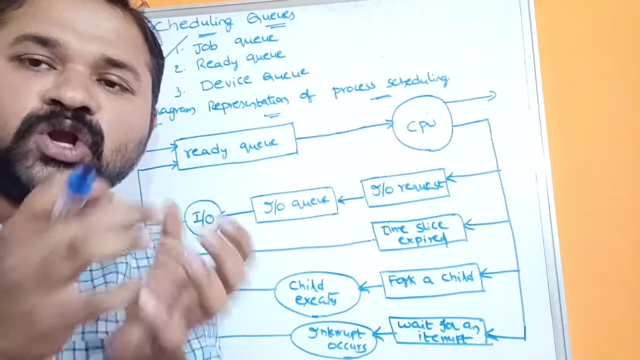 We know that CPU can execute. So the CPU can execute the process If it resides in main memory only. So if the process resides in main memory, then only CPU executes the process. So the operating system loads the processes from secondary memory to main memory. 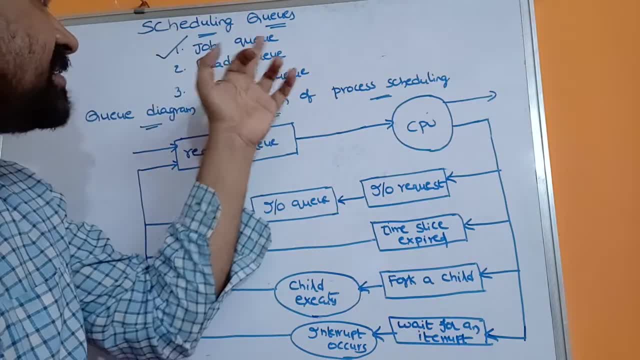 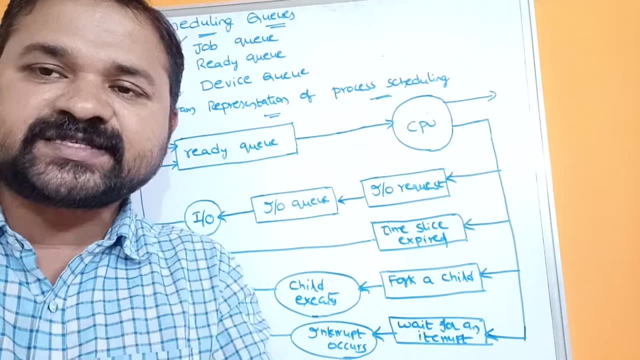 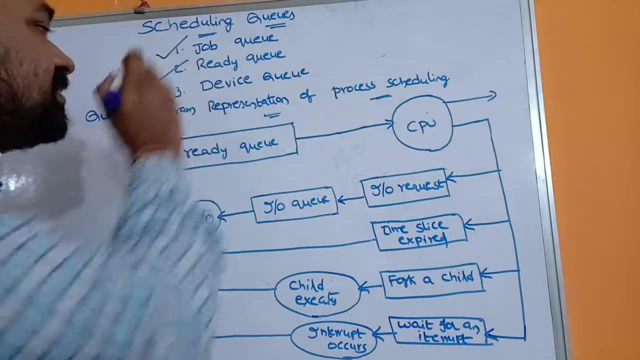 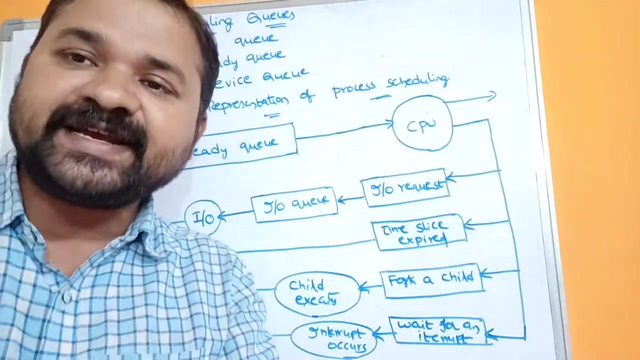 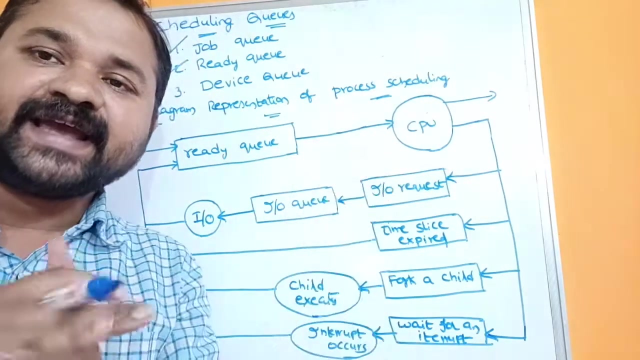 Those processes will reside in ready queue. So what is ready queue? It contains a list of processes, list of processes which are ready for execution by the CPU. so where ready, you will recess. ready, you will resides in main memory. various job, you will resides in secondary memory. and the next one is device Q. device Q contains a list of 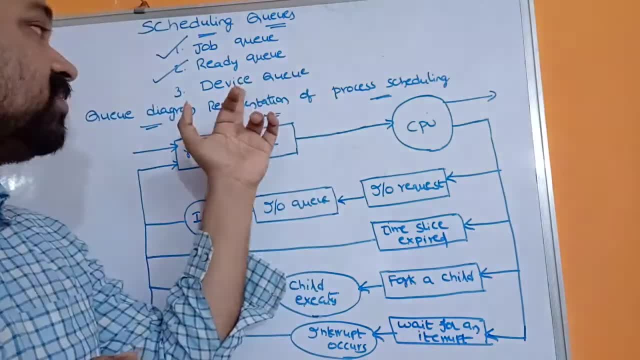 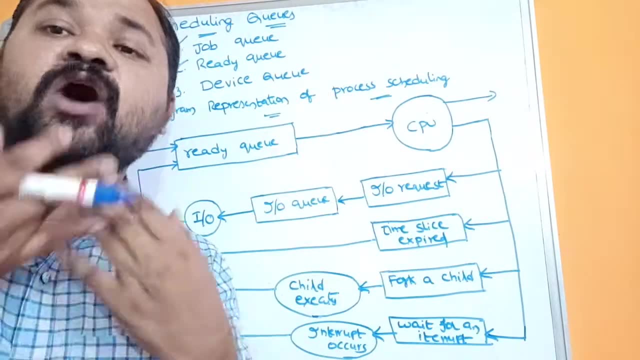 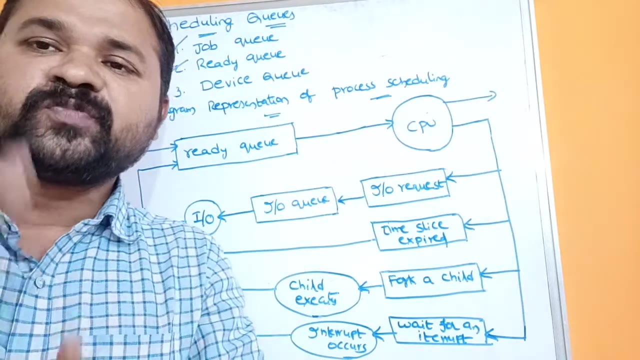 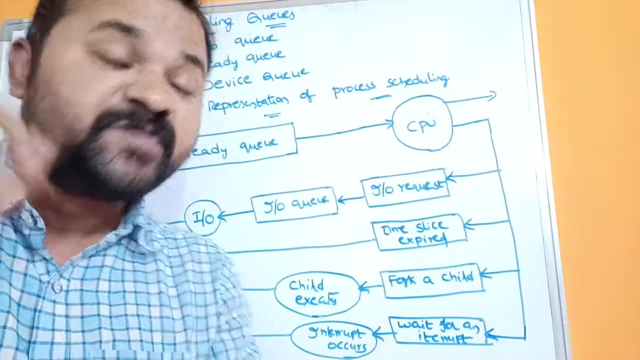 processes which are waiting for an Ivo operation. here device means it may be either input device or output device. we know what is input operation. input means reading data from the file where he has. output means citing data into the file. let a process is waiting for some Ivo operation, then the corresponding process. 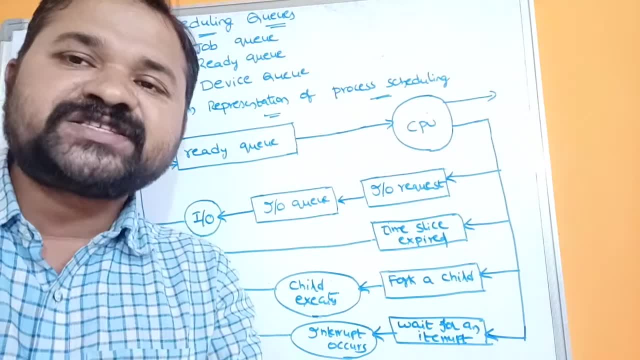 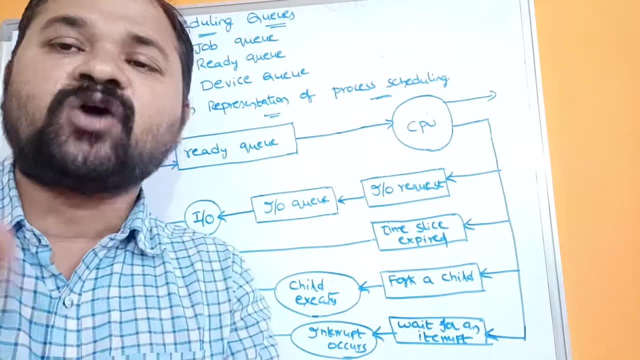 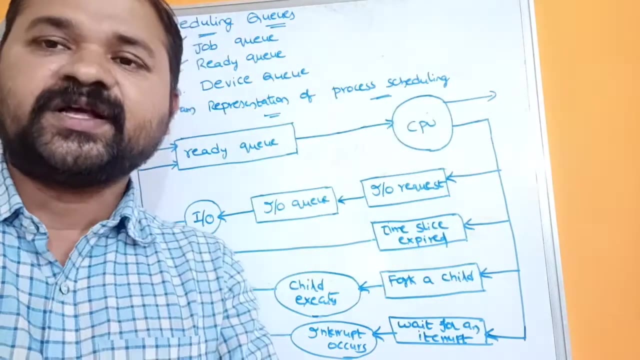 will be put it device Q. okay, so device Q contains a list of processes which are waiting for input- output operation. it may be any operation. it may be some input operation or output operation. it may be any operation. if a process is waiting for any operation, then the corresponding 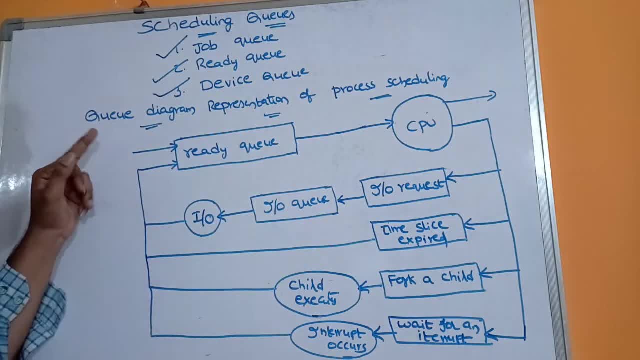 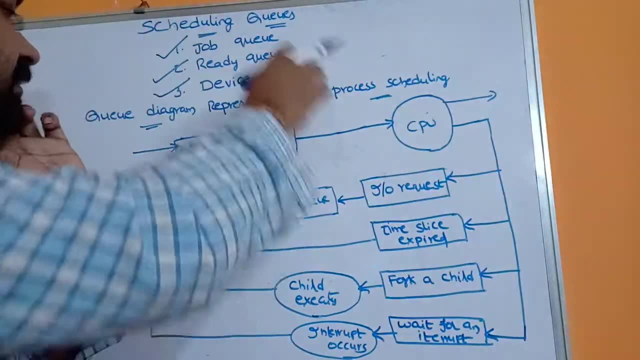 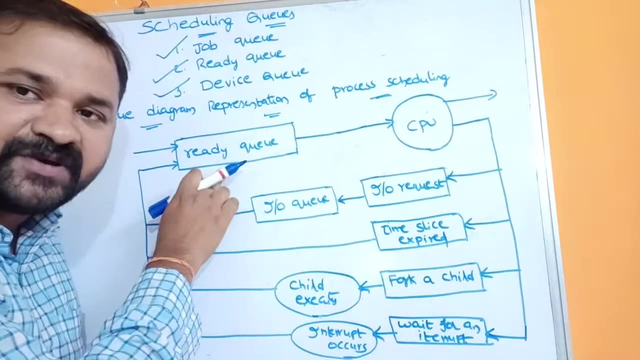 process will be putting device Q. okay, now let's see the Q diagram representation of process scheduling. so how we can draw the process scheduling diagram diagram you will be able to dum зм some use here we are maintaining to use the first active is radical, we everyday. second, Q is I want you here we are not. 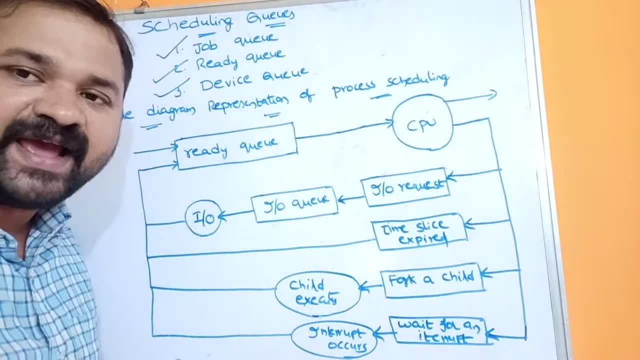 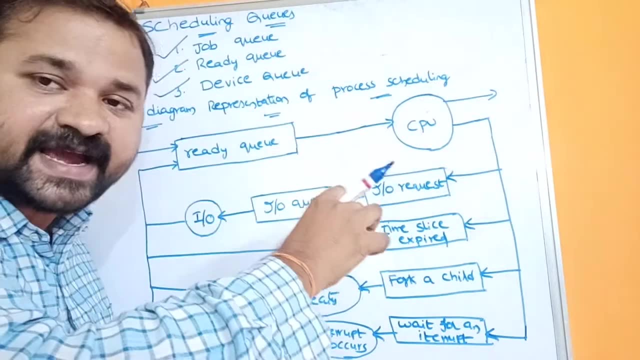 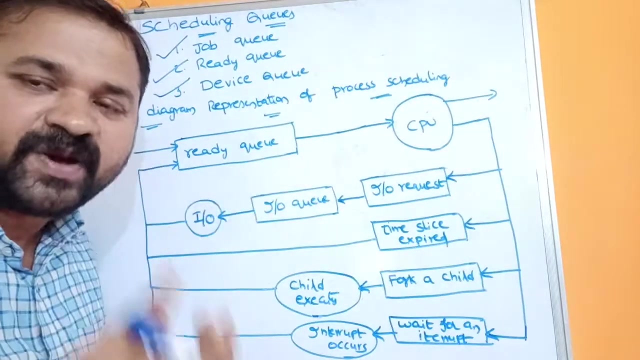 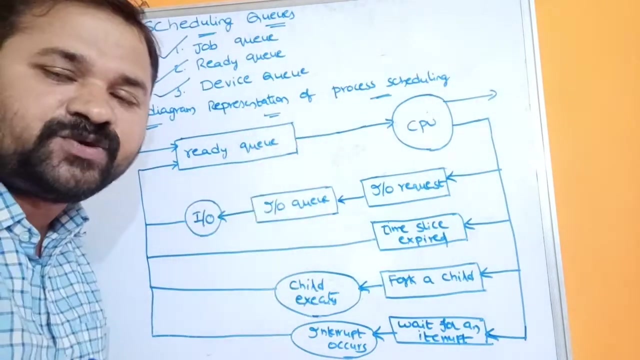 maintaining any job you. so, first of all, we have it: operating system modes, the missions processes from secondary memory to the main memory. those processes will be an Arabic. you, that means operating system logic. Contığı that the I AM pizza host of Antec, the processes from job queue to the ready queue. okay, so what is ready queue? ready queue contains: 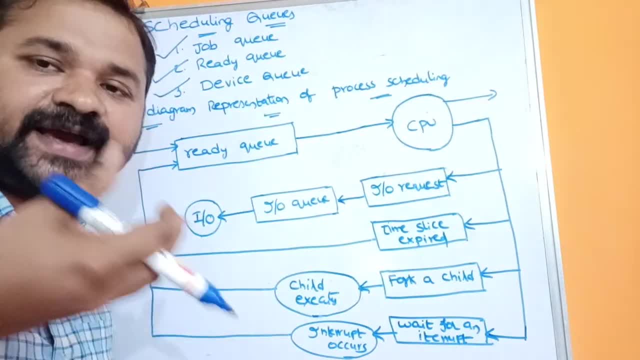 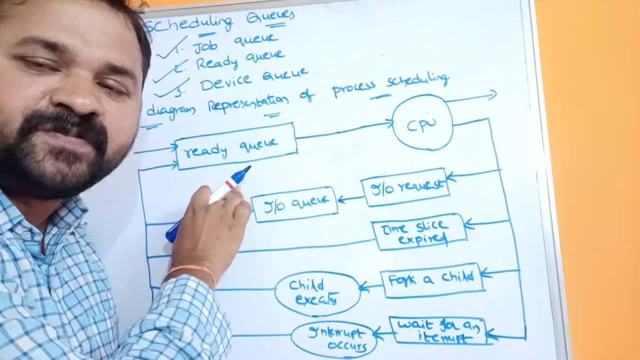 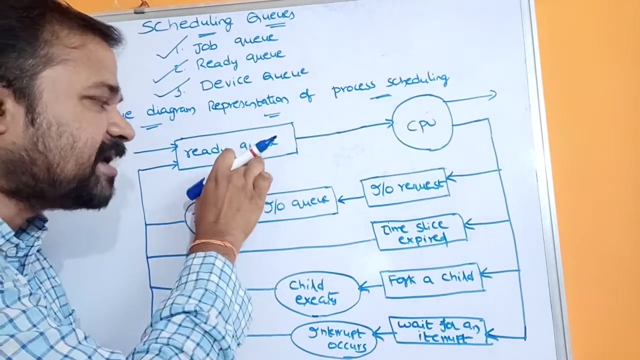 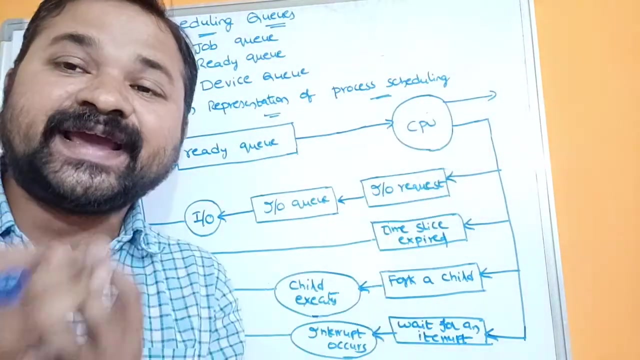 a list of processes which are ready for execution by the cpu. so whenever cpu is free, then operating system allocates cpu to the process. so operating system picks one of the process from the ready queue and allocates cpu to that process. so now cpu starts execution of that process. okay. 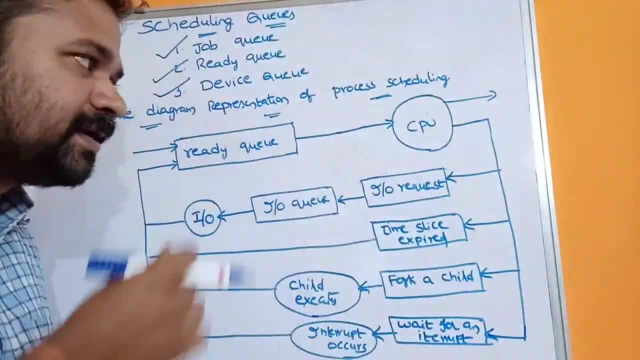 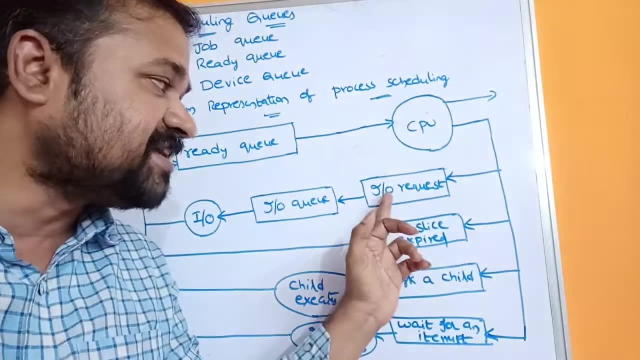 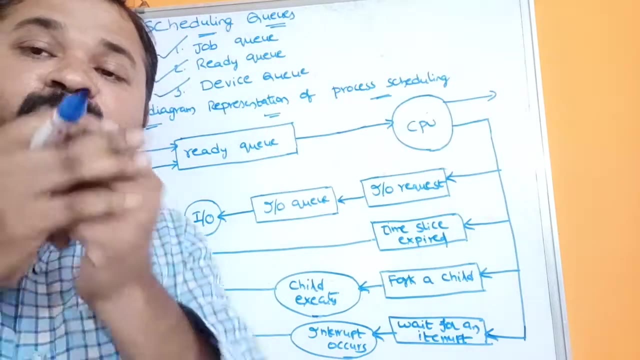 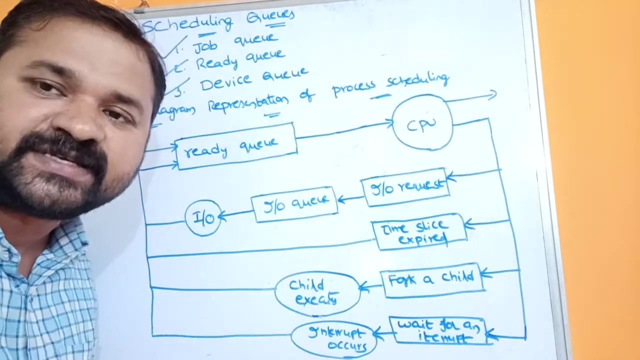 why cpu is executing that process assumes that a process is waiting for some ivo operation, so that request is known as ivo request. so if a process is waiting for an ivo operation, then that process has to be moved to the ivo queue, because ivo queue contains list of processes which are waiting for ivo operation. 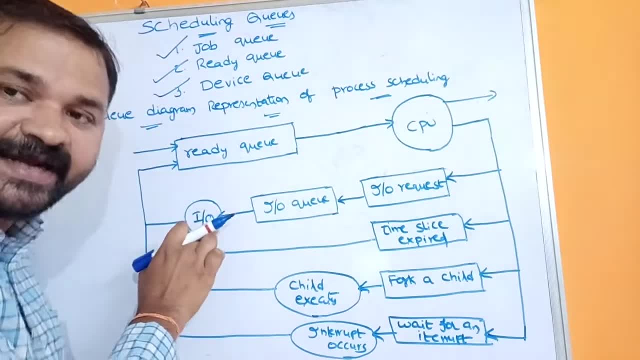 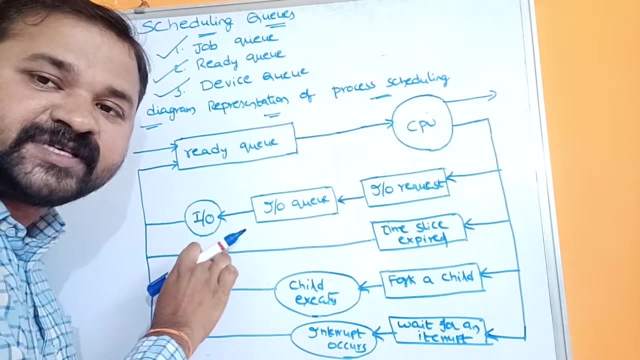 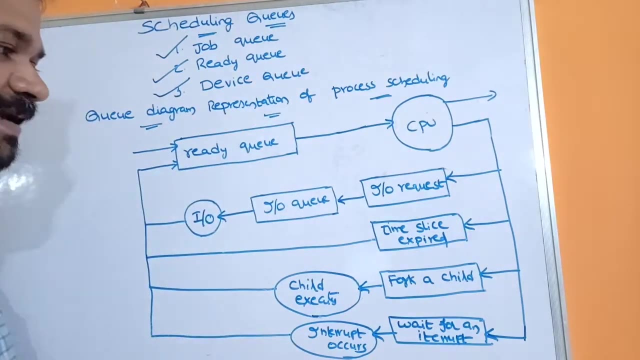 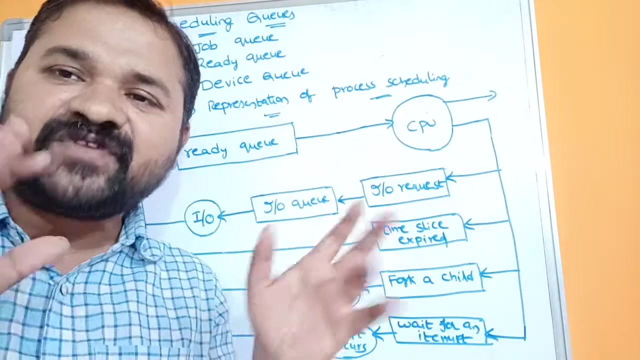 so once that ivo operation is completed, once that process has completed its ivo operation, then the corresponding process is ready for execution. so the corresponding process will be moved to the ready queue. okay, and let's see the next scenario in a. here we have different scheduling algorithms. here we have a scheduling algorithm called 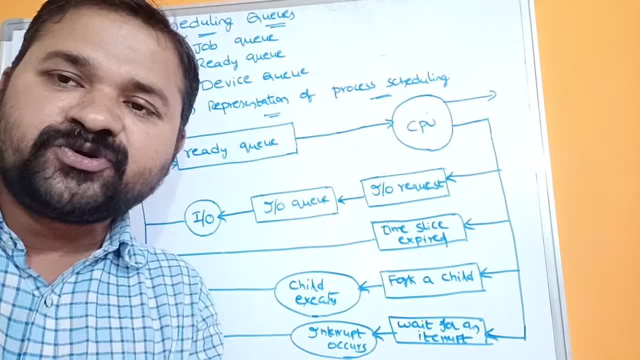 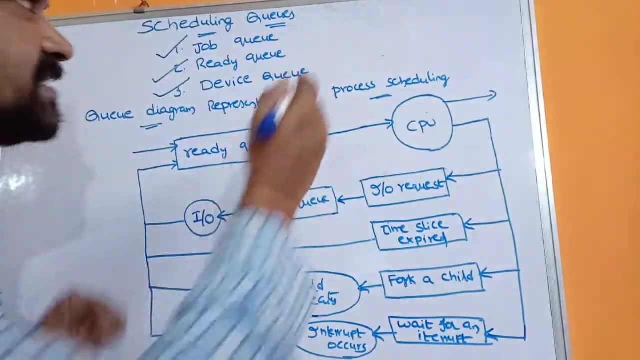 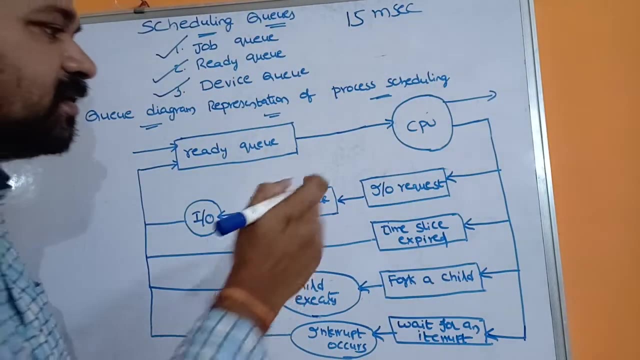 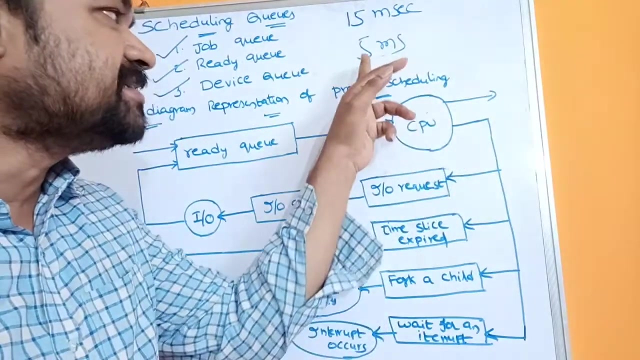 round robin scheduling algorithm. in round robin scheduling algorithm, a process will be executed for a particular time slice period. let us assume that a process requires 15 milliseconds of time for its execution, whereas the closest time quantum is 5 milliseconds. so cpu is executing that process here. what is the time quantum? 5 milliseconds is the time slice. 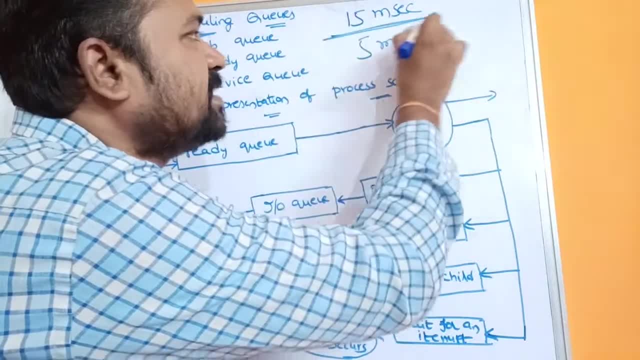 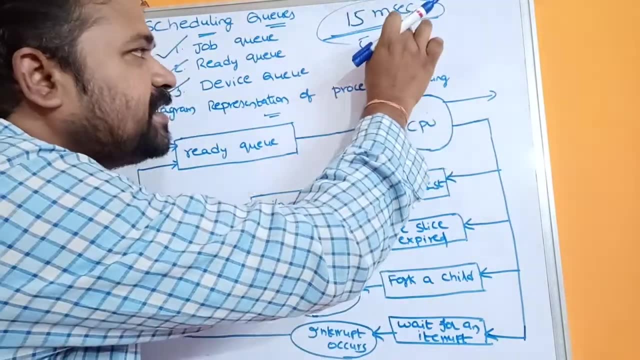 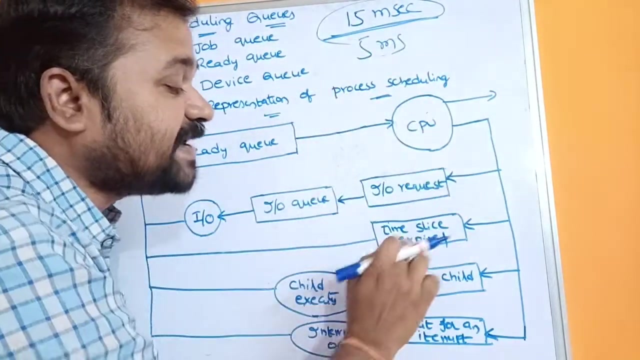 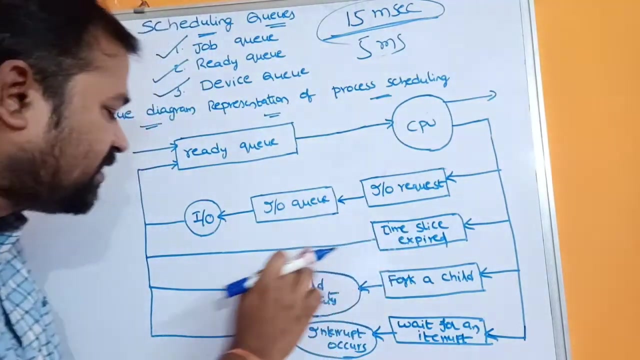 period, whereas the process requires how many milliseconds? 15 milliseconds- in order to complete its execution. okay, so here cpu is executing this process. so cpu executes the process for 5 milliseconds if that time slice period expired. if that time slice period expired, then the corresponding process will be moved to the ready queue. so the remaining 10 milliseconds of 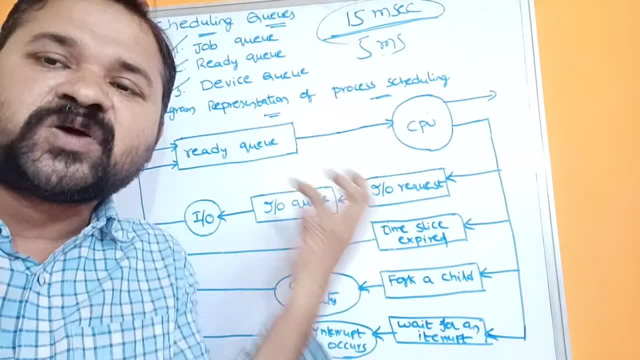 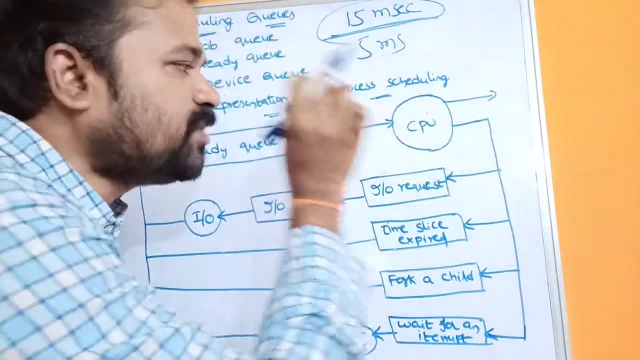 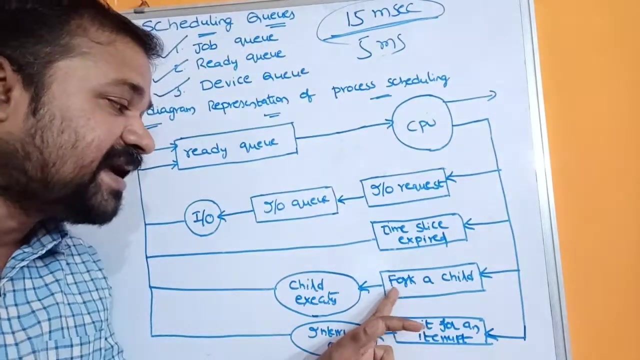 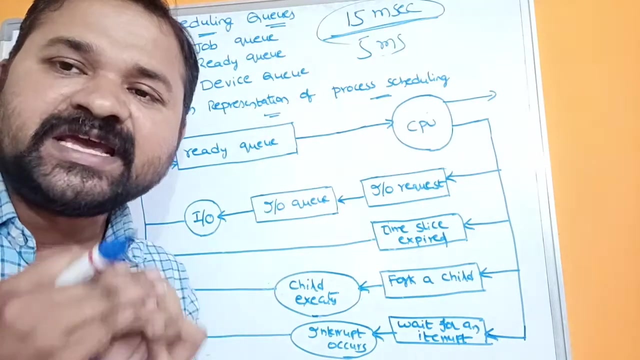 time will be executed later. that depends upon the operating system. okay, and let's see the next scenario, why cpu is executing the process assumes that a process produces its child with the help of fork function. here we have a function called function. fork function is mainly useful in order to produce a child process. okay, so while cpu is, 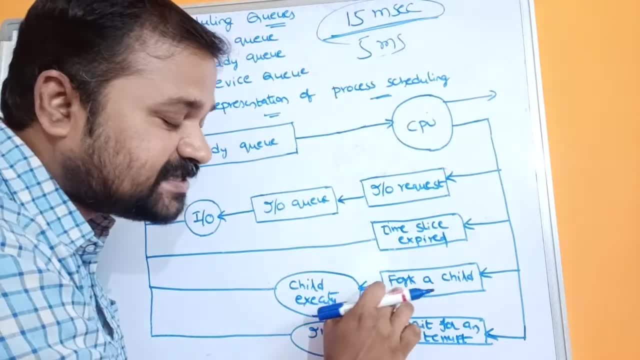 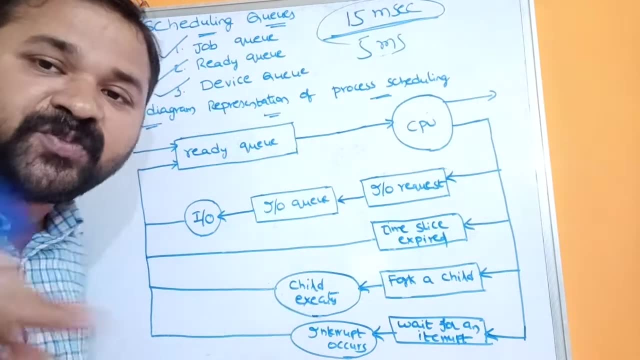 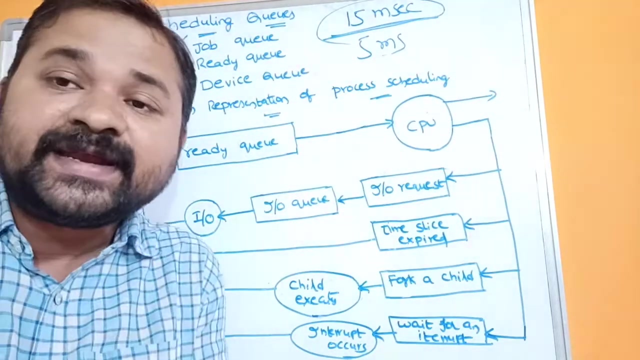 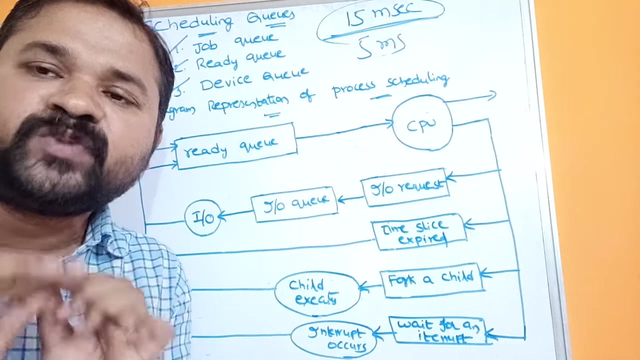 executing a process, then that process produces a child with the help of fork function, then the corresponding child process has to be completed, its execution. so if the child process is completed its execution, then it is moved to the ready queue. so first the child process has to be completed, its execution. so once its child process execution, 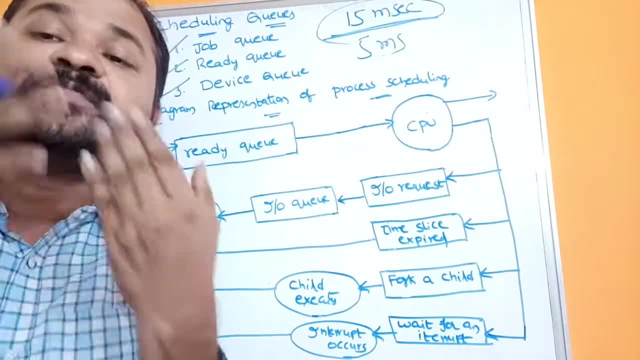 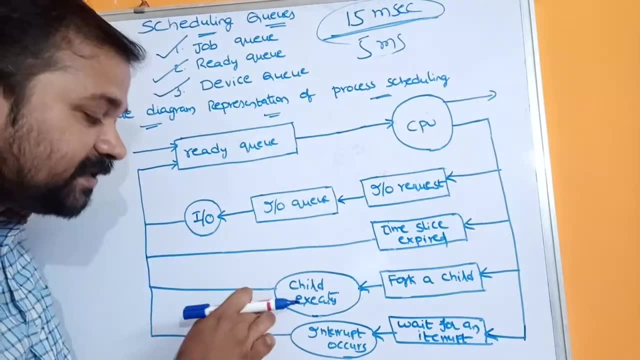 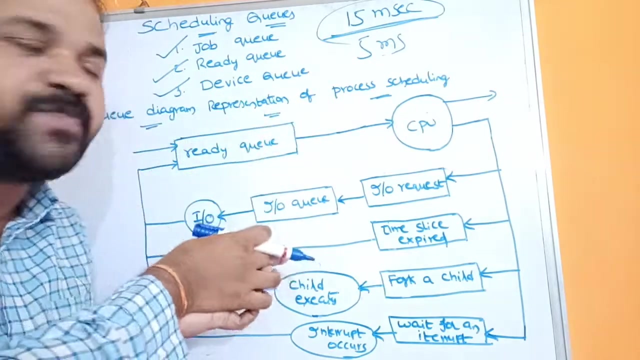 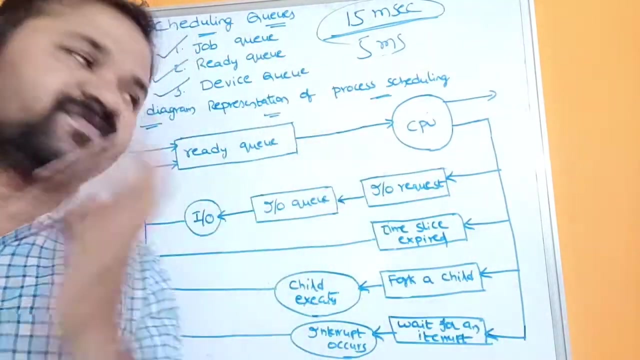 is over, then remaining instructions of that parent process will be executed. okay, so once channel process execution is over, then the corresponding process will be moved to the ready queue. then after some time, operating system allocates that process to the cpu. so cpu starts execution of the remaining instructions from where it is left. okay, so life is here also okay. 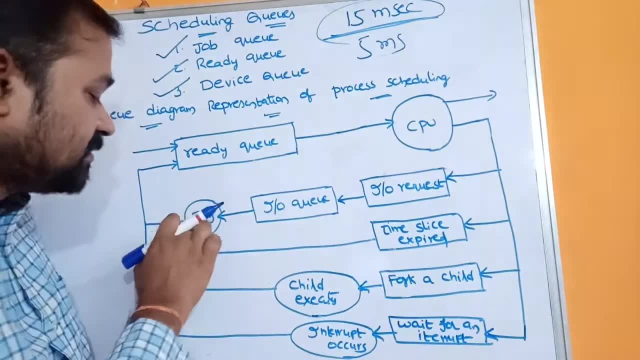 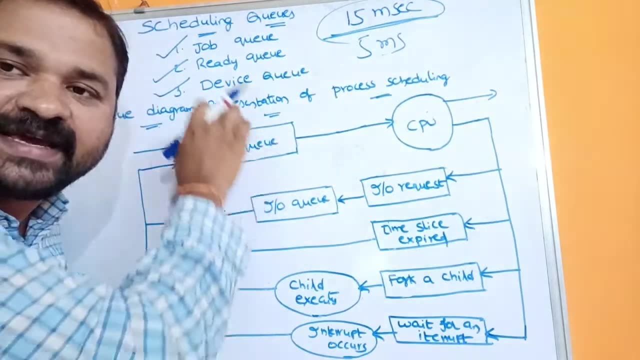 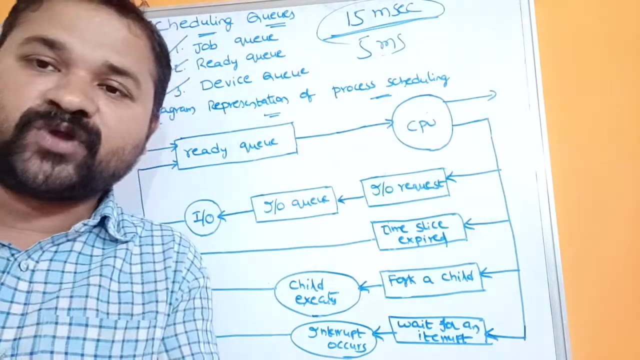 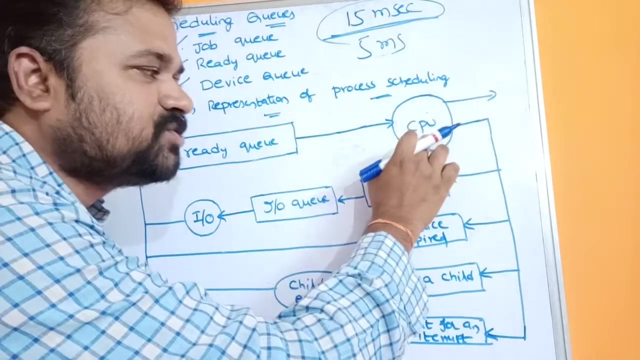 whenever that process completed its i o operation, then the corresponding process will be moved to the ready queue. so after some time, operating system allocates cpu to that process. so cpu starts executing the remaining instructions of the program. okay, from where it was left. okay, and let us take one more scenario. let us assume that cpu is executing a process. so why cpu is? 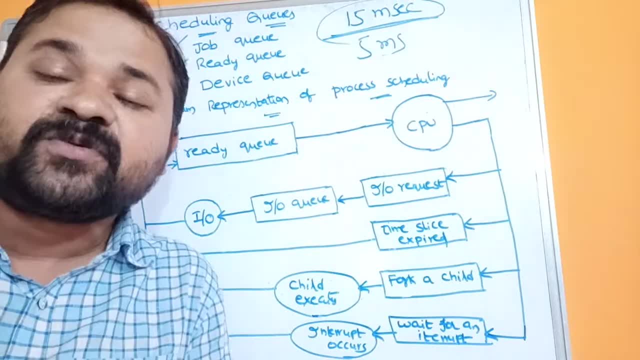 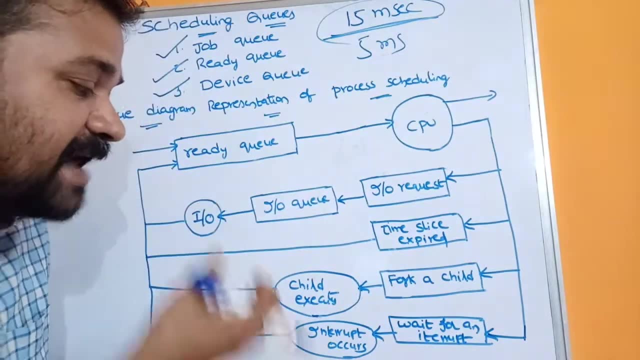 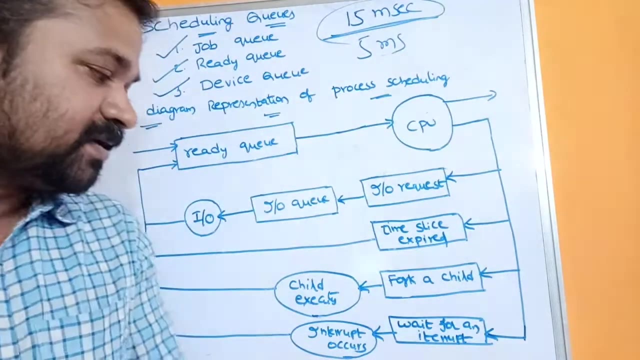 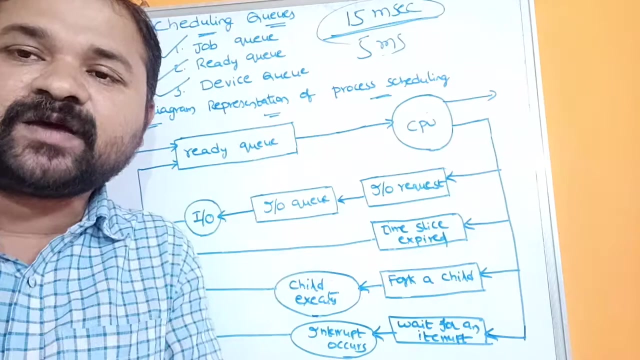 executing a process, it receives an interrupt from the operating system. it receives an interrupt from the operating system. so once an interrupt occurs, okay, then the corresponding process has to be moved to the ready queue. okay, so it is waiting for some interrupt. so whenever that process, whenever that cpu receives an interrupt, so that process will be moved to the 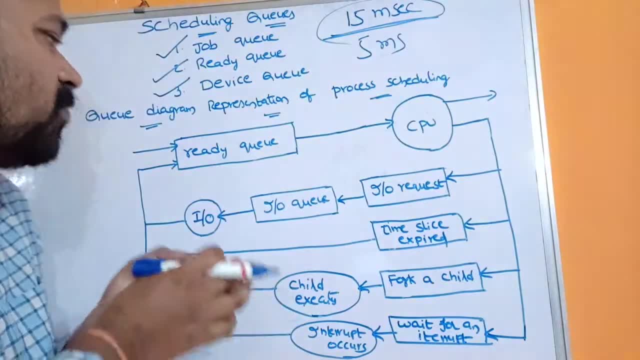 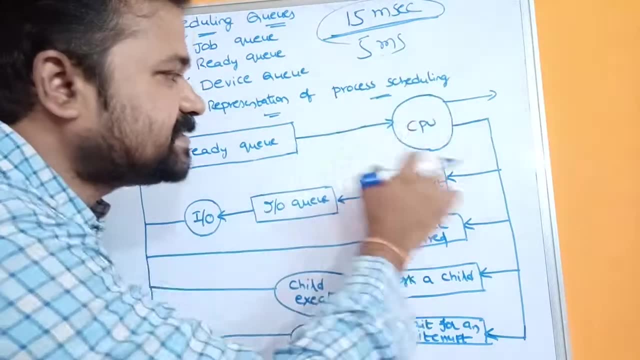 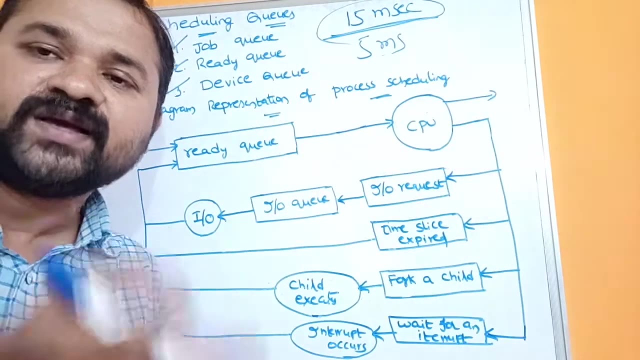 ready queue. so after some time, operating system allocates that process to the cpu. okay, here let us observe this diagram here. this is nothing but cpu time. this is nothing but i? o time we have. every process is represented with the help of cpu time and i o time cpu burst to process, i o. 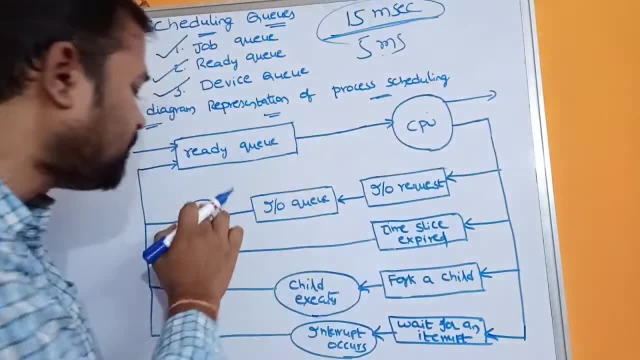 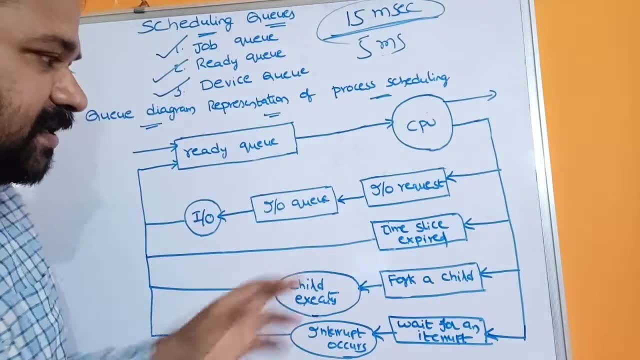 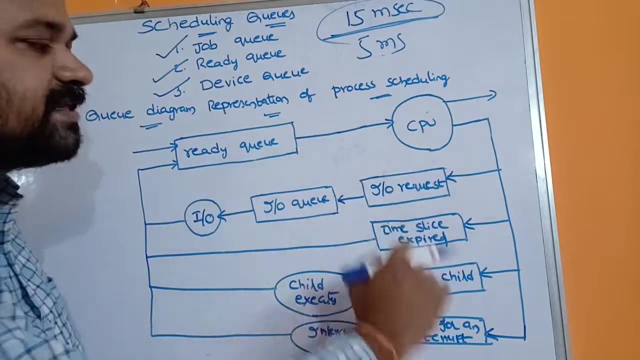 burst to process like that. here we have to represent cpu and i o with the help of a circle, next ready q and i o q. so next i o request time slice, exploit 4k child, wait for an event, wait for an interrupt. so all these are to be. 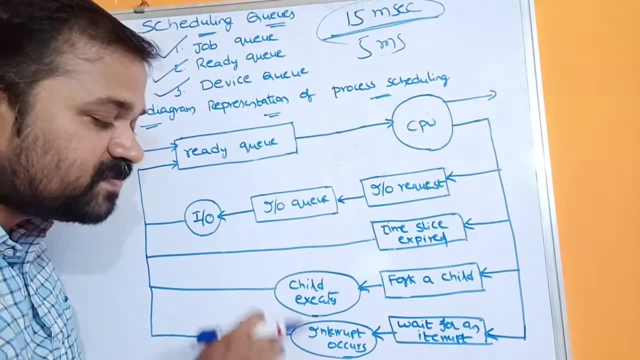 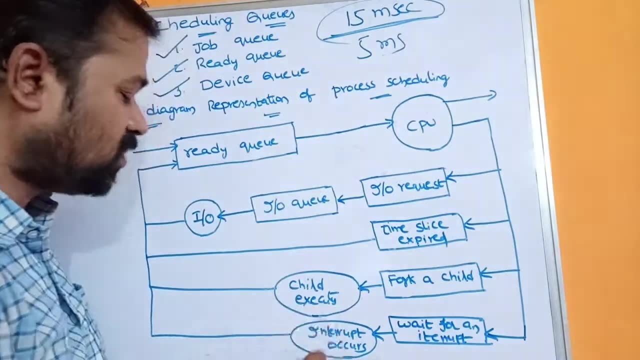 represented within the rectangle, whereas these are nothing but some events, some actions. so, whenever child execution is over, whenever an interrupt occurs, these, these two are to be represented within some ellipses like that. so, whenever an interrupt occurs, these, these two are to be represented within some ellipses like that: 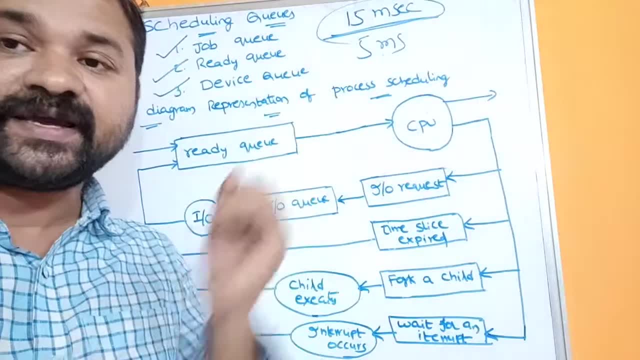 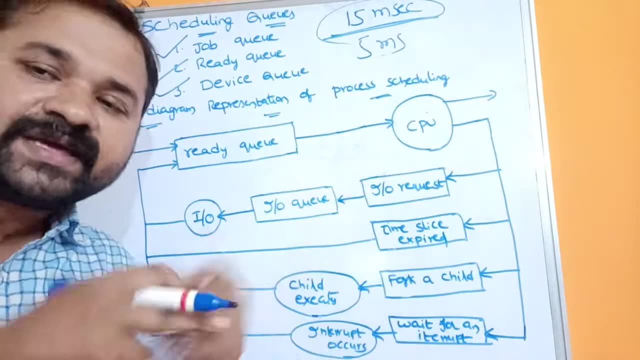 okay, so this is about scheduling queues, okay, so mainly we have three types of queues: job queue, ready queue and device queue. and this is nothing but queuing diagram for the process scheduling.